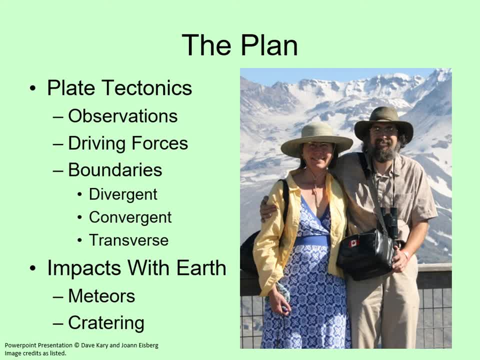 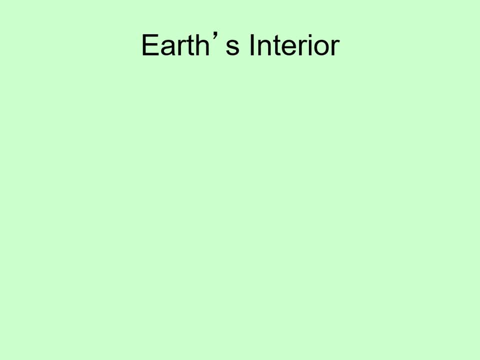 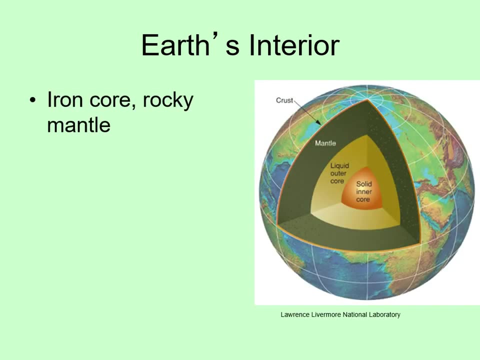 As we'll see, the largest of these could even have affected the evolution of life. Let's start our look at the Earth's surface by reminding ourselves of what the interior is like. The Earth is divided into a two-layer iron core surrounded by a thick mantle made of rock. 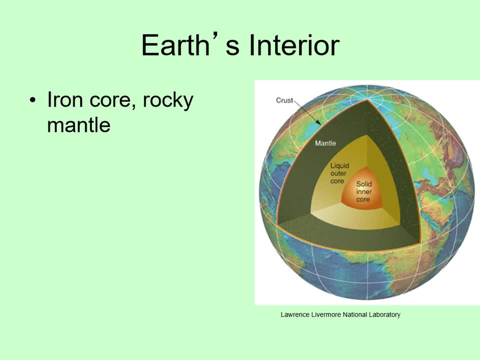 The outer core is hot liquid iron. The inner core is even hotter, but the greater pressure squeezes the iron to a solid. The mantle is also mostly solid, but the inner core is even hotter. The mantle is also mostly solid, but the inner core is even hotter. but the greater pressure squeezes the iron to a solid. 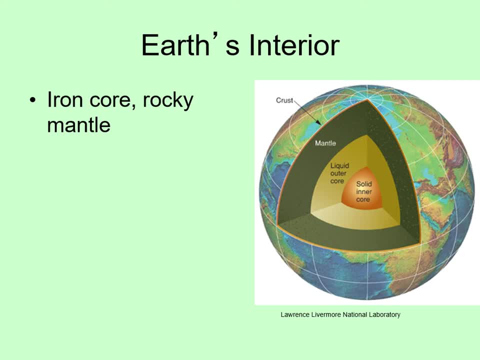 The mantle is also mostly solid, but the inner core is even hotter. but the inner core is even hotter At these tremendous pressures and temperatures. even rock flows very slowly. only a few centimeters per year. This is about the same speed fingernails grow Because of this slow, fluid motion. 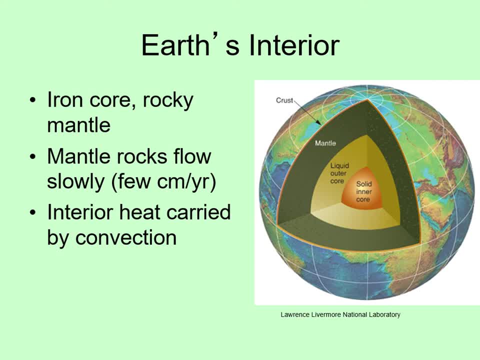 the mantle carries heat through convection. Hot mantle rocks flow upward from the interior, while cooler rock sinks back down towards the core. The crust we live on floats on top of this solid rock. The mantle carries heat through convection. The hotter the rock, the slower it sinces back down from the interior. 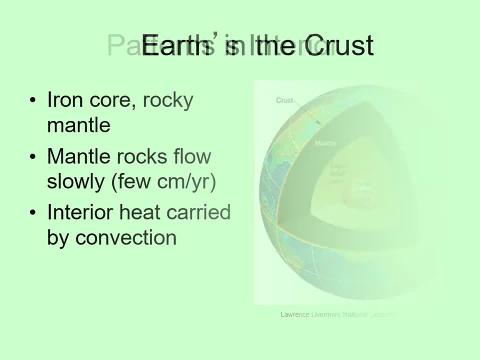 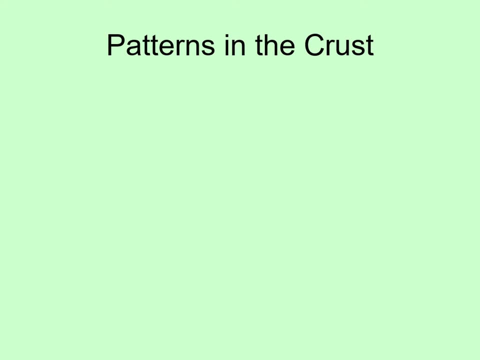 slowly overturning mantle. Now let's look at the crust We're going to focus on where we see volcanism and tectonics on the Earth's surface. As we'll see, geological activity doesn't just happen randomly on the Earth. 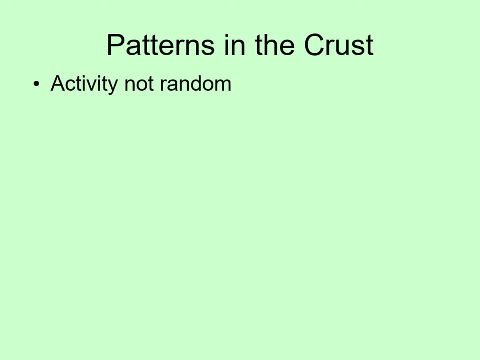 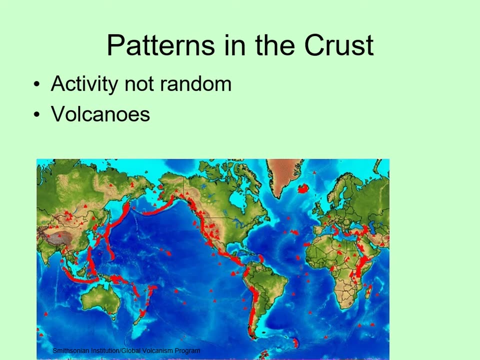 The pattern of how it is distributed gives us important clues that lead to plate tectonics. Here's a map of the Earth's major volcanoes. Notice that most volcanism happens along thin lines, mainly at the edges of continents. There are very few volcanoes in the middle of continents. 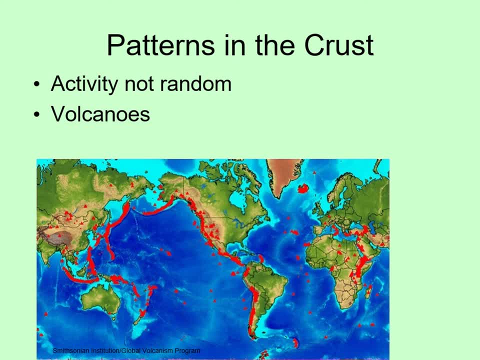 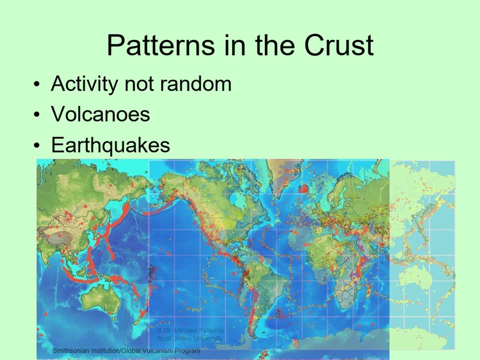 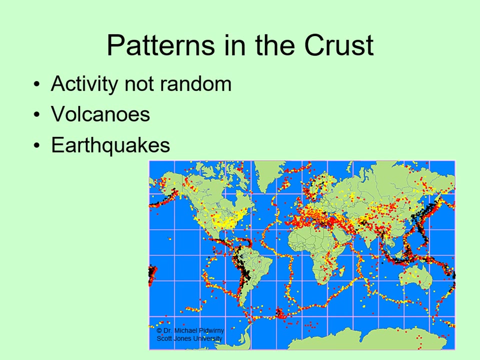 Note that this map leaves out the ones at the bottom of the ocean. The ones you see in the oceans are all on islands. Now compare this with a map of where earthquakes occur. Remember that earthquakes are a sign of tectonic activity on the surface. 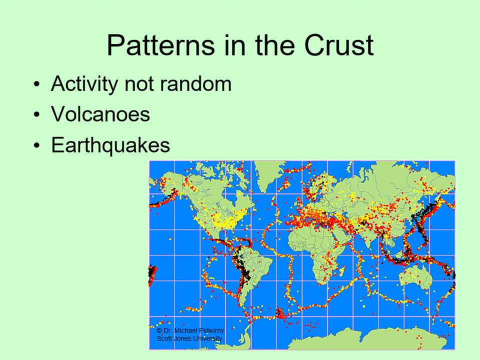 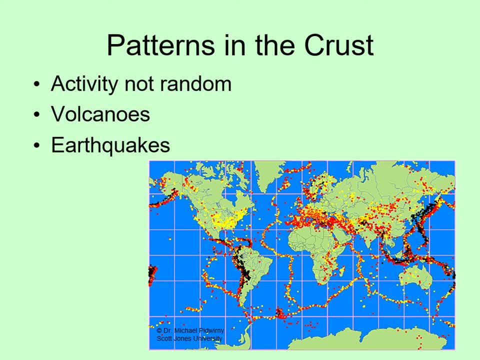 though here we also see many of the quakes that happen in the oceans, also along narrow lines. The key observation here is that these two sets of data overlap. Volcanoes and earthquakes happen in many of the same places, and these places mark out the edges of large, stable regions with much less activity. 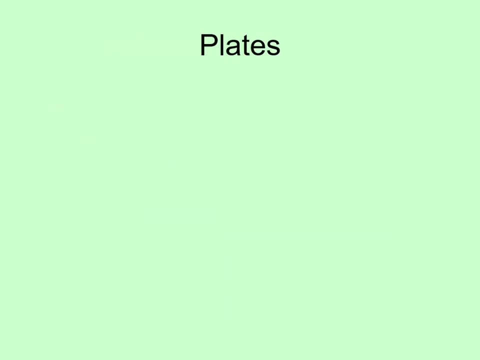 this leads us to the concept of crustal plates. the idea is that the earth's crust is broken up into a series of rigid sections called plates. the central parts of these plates are relatively stable, so they show few signs of volcanic or tectonic activity. however, the places where 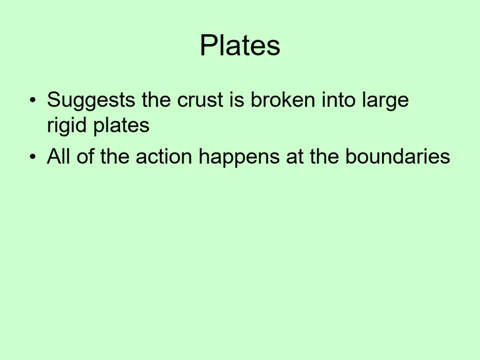 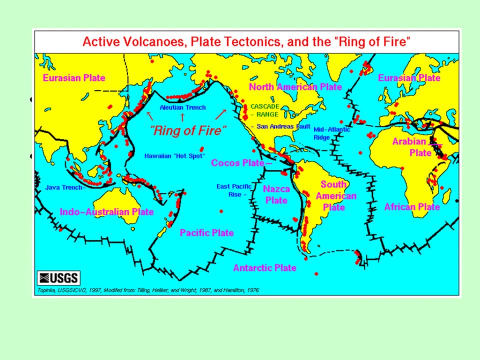 plates meet are a different story. these plate boundaries are where the geologic action is. this map shows the major plates that make up the crust. the thick black lines mark the plate boundaries and the red dots are active volcanoes. notice that there are huge plates, like the pacific and north american plates, along with much smaller ones like the cocos plate off. 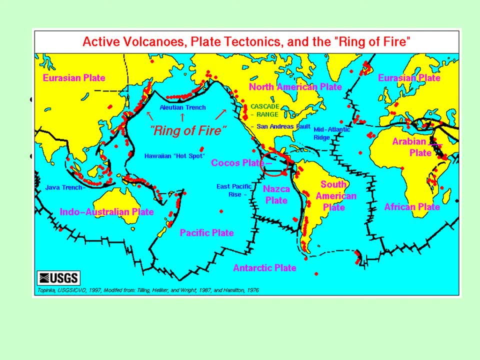 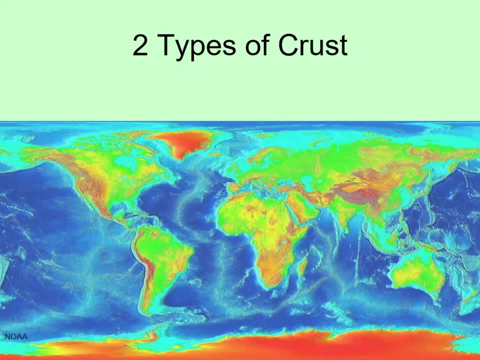 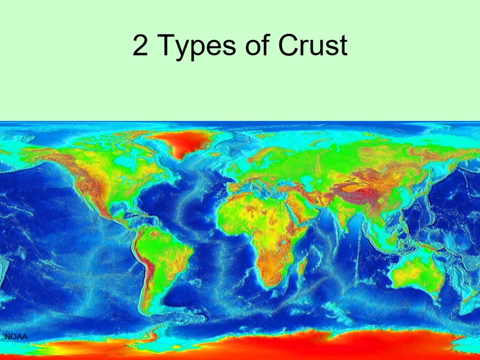 of central america. there are even some smaller ones that aren't labeled here, like the ones offshore from the cascades range. have a look at this map of the world. with the oceans removed, you can still make out the shapes of the continents, although they do look a little distorted. there isn't a smooth transition from continent to ocean bottom. 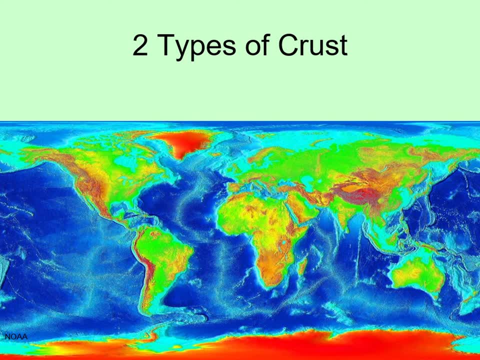 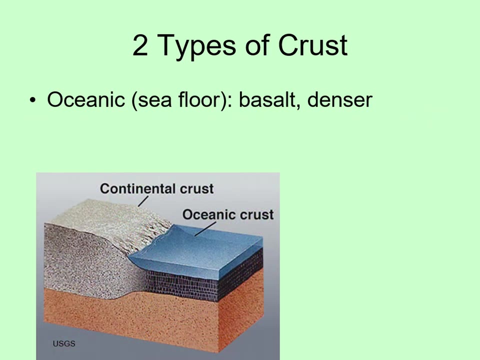 instead, there's a relatively steep drop off just offshore from the continental edges. this reflects a real difference in the composition of continental and oceanic crustal rocks. oceanic crust: once you get below the sand and silt, there's no clue how to get below the sand, so just stay with these passes. 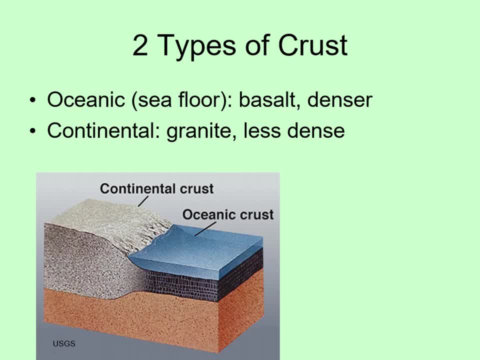 so these grow in the sand and the rocks are from east coast. some of thesta big rocks show the locked lake. one of these rocks is called Ba Gramate. it's a spine like rock and is denser to the sea. larger Legrandite rock. 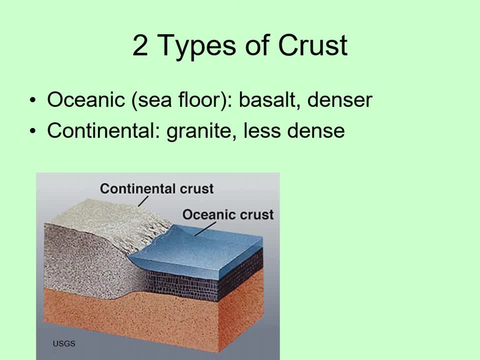 the northern sign, the northernァ 엑 small rock, the northern Mitsunay rock is thin and hopes going forimetahren uto little more. going forimetrain, with a deeper funk stick up several kilometers higher than the oceans, Those drop-offs at the edges of continents. 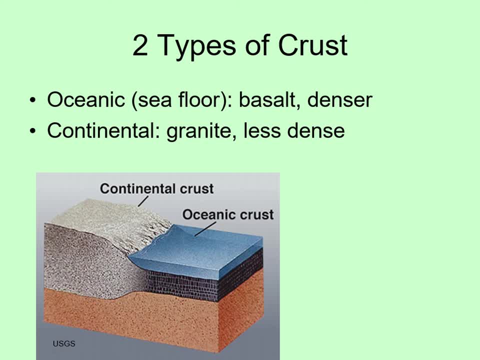 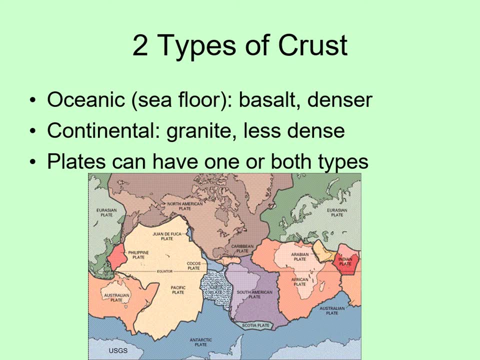 mark the boundaries between the two types of rocks. So notice that some plates are virtually all ocean, like the Pacific plate, while others have a mixture of continent and ocean. Look at how the North American plate extends out to the middle of the Atlantic Ocean. 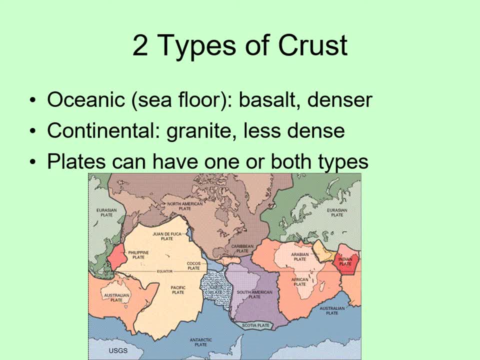 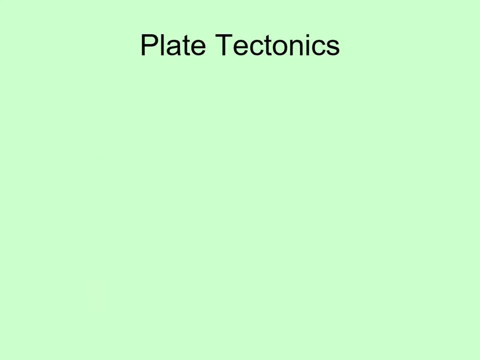 The drop-off from continental to oceanic rock happens within this plate, So one plate can have two kinds of rock Plate. tectonics is the motion of these crustal plates. We should think of the crust as floating on top of the denser mantle. 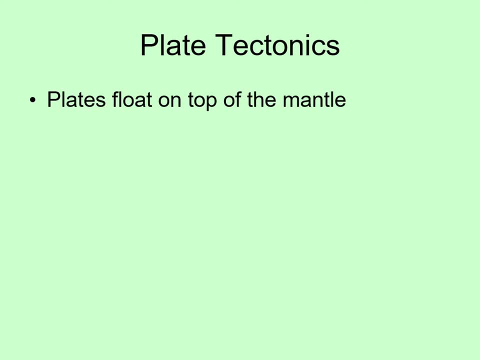 Remember, the mantle is undergoing a slow convective motion. Hot mantle rocks rise and cooler rocks sink, creating a constant overturning motion. The crustal plates are dragged along with this flowing mantle, with new plates rising and new plates falling, New plates forming in some areas. 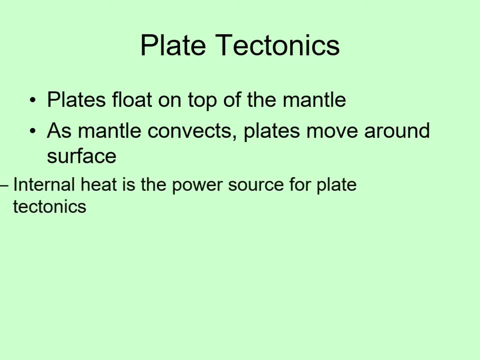 and old ones dragged back into the mantle in others. So the power source behind plate tectonics is the Earth's internal heat, causing the mantle to flow. There are three major types of plate boundaries. The first is a divergent boundary. 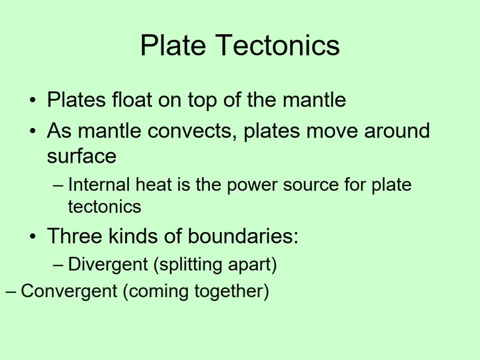 This is where two plates are pulling apart. The next is a convergent boundary, where two plates are squeezing together. The last is a transverse boundary, where two plates slide past each other. Let's look at each of these in detail. At a divergent boundary: 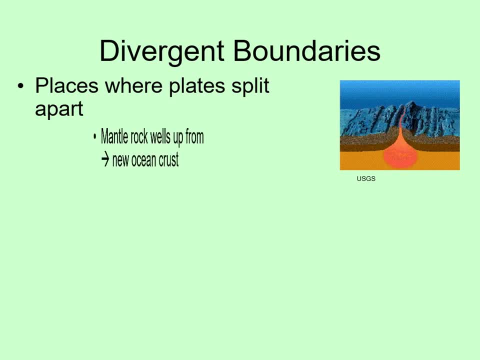 two plates are pulling apart from each other. This happens at the places where hot mantle rocks are coming up from deep inside the Earth, So the mantle rocks squeeze up between the plates and create new crust on the edge of each plate When this mantle solidifies. 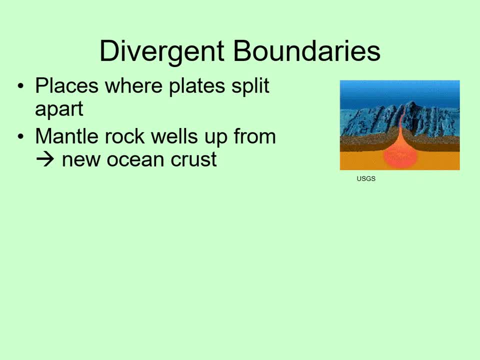 it produces basaltic rock, So the new crust that forms is oceanic crust. The most common kind of divergent boundary on the Earth is a mid-ocean ridge. These are long mountain ranges running through most of the world's oceans. 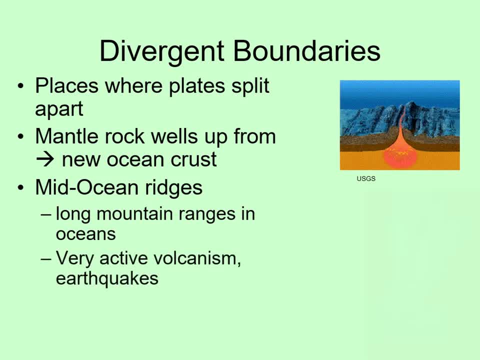 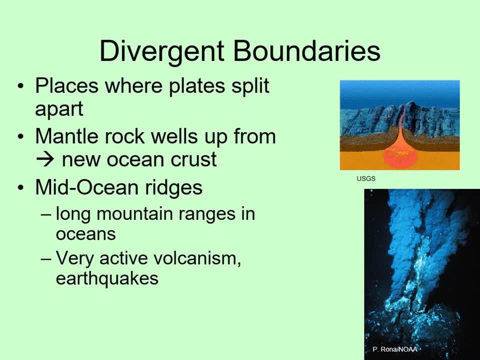 They form from the upwelling mantle and they show many volcanic features, like this black smoker underwater volcano. There are also many earthquakes along these boundaries. This map shows part of the Atlantic Ocean, with the mid-Atlantic ridge running down the middle of it. 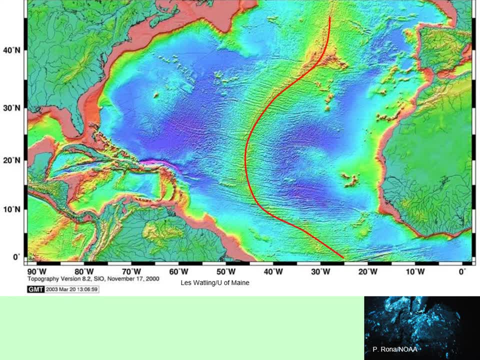 This map shows part of the Atlantic Ocean, with the mid-Atlantic ridge running down the middle of it. Notice that it bends to follow the shapes of the coastlines on either side of it. Notice that it bends to follow the shapes of the coastlines on either side of it. 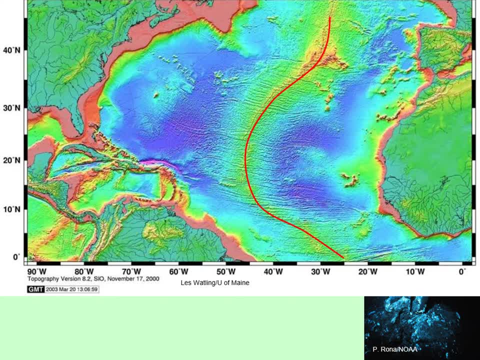 Notice that it bends to follow the shapes of the coastlines on either side of it. Mid-ocean ridges and their surroundings. Mid-ocean ridges and their surroundings were some of the first features that truly convinced geologists that plate tectonics was a good description of the Earth's geology. 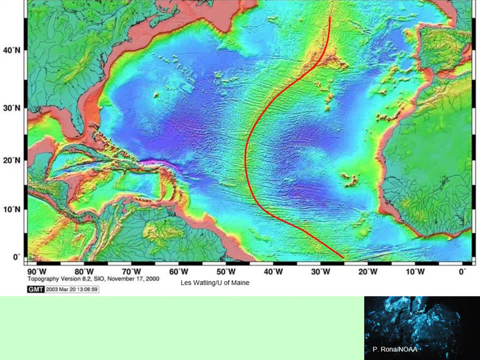 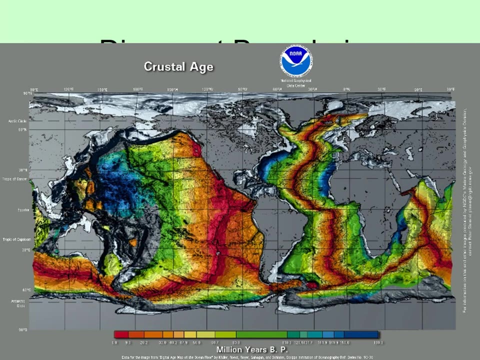 This happened because geologists noticed that the age of the ocean crust follows a very special pattern Along the ridge. the crust is always very young, getting progressively older as you move away from it. In this global map of the oceans, you can see that it's a very symmetric pattern on either side of the ridge. 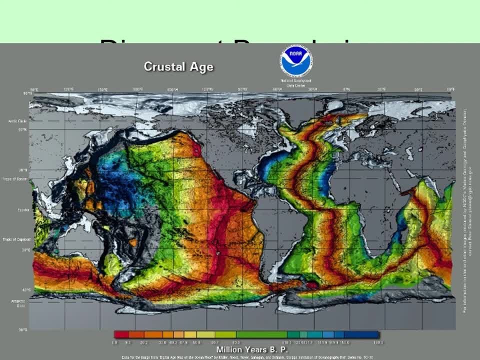 Clearly the ocean crust has grown from the locations of the ridges spreading outward in either direction. Notice something else about this map of ocean crustal ages: The oldest part of the ocean crust shown in dark blue is less than 200 million years old. 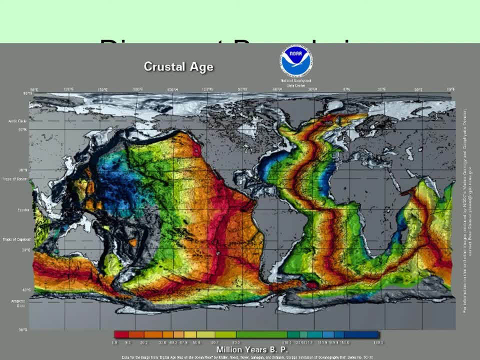 In comparison with the over 4 billion year age for the Earth as a whole, this is a very short time. On many parts of the continents, it's not unusual to find rocks that are hundreds of millions to a couple of billion years old. 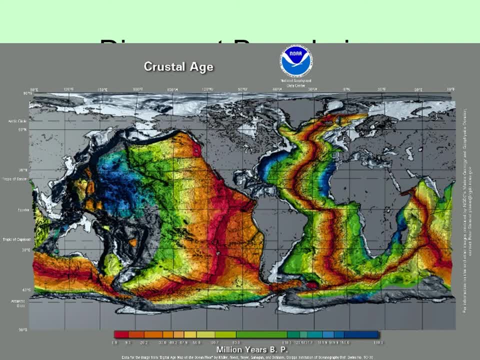 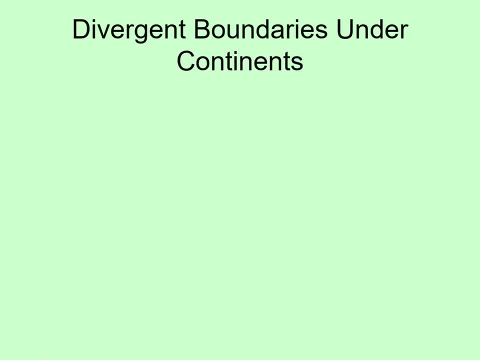 So the ocean crust is clearly disappearing just as fast as it's being formed. We'll come back to this observation shortly. Sometimes the mantle upwelling happens under a continent instead of in the middle of the ocean. When this happens, the continental crust begins to thin and eventually split apart. 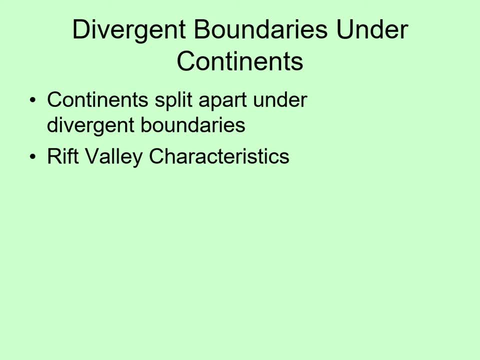 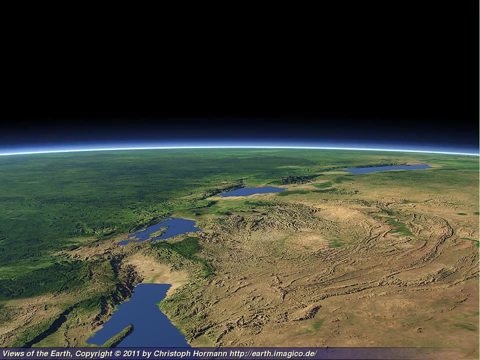 This creates a feature called a rift valley on the continent. These are characterized by active volcanoes, long narrow valleys and lots of earthquakes. The best example of this on Earth at the moment is eastern Africa, where a set of rift valleys extend along much of the eastern half of the continent. 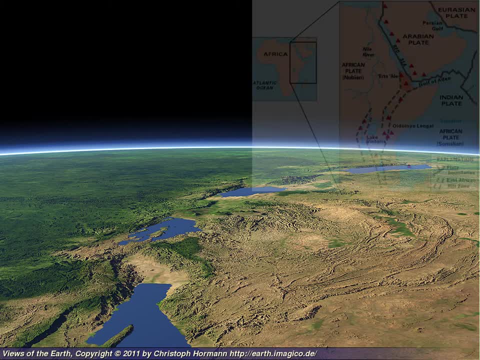 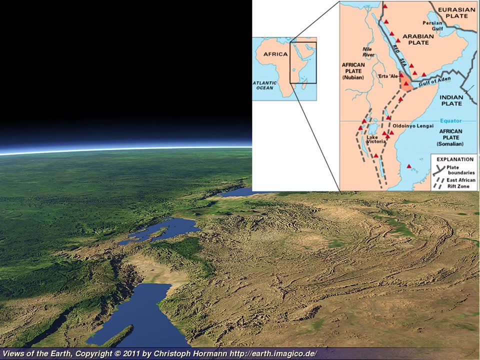 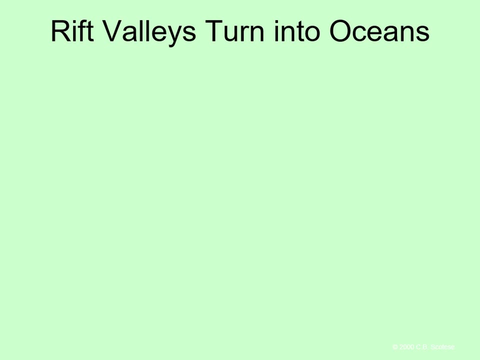 threatening to split eastward. This is the case for the northern half of the continent, where the Red Sea divided the Arabian Peninsula from northeastern Africa. Using a variety of clues, geologists have plotted out the motions of the Earth's crust over the last several hundred million years. 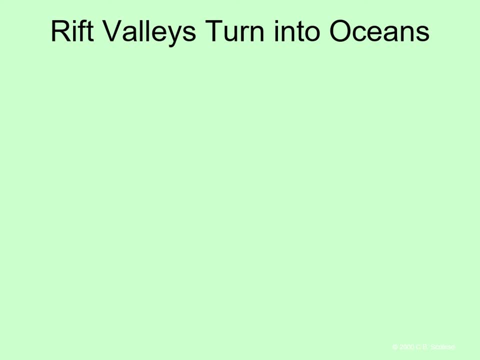 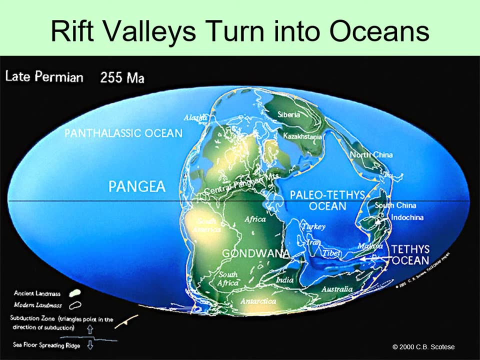 And this shows how rift valleys have evolved into oceans over time. 255 million years ago, the Earth's major continents were all joined together. Some areas that are now joined together into a single supercontinent we call Pangea. Some areas that are now joined together were widely separated. 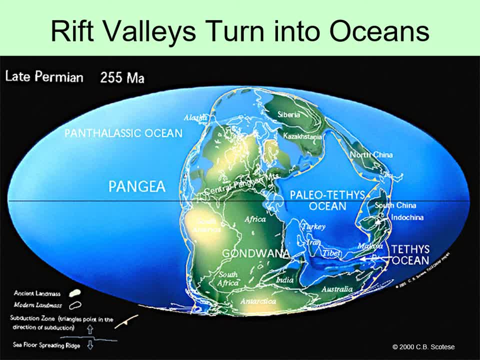 and some areas that are now land were covered with shallow seas, like western North America. in the upper part of this map, Pangea wasn't the first supercontinent, but it's the one we can piece together most easily because it was the most recent one. 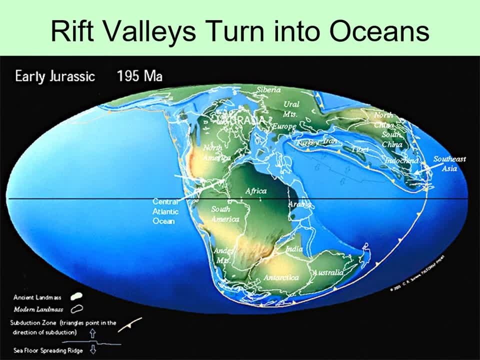 By 195 million years ago, early in the era of the dinosaurs, much of Asia had split off from the rest to form an early version of the Indian Ocean. Notice that India was wedged in next to Africa and a new mountain range was developing along the west coast of North America. 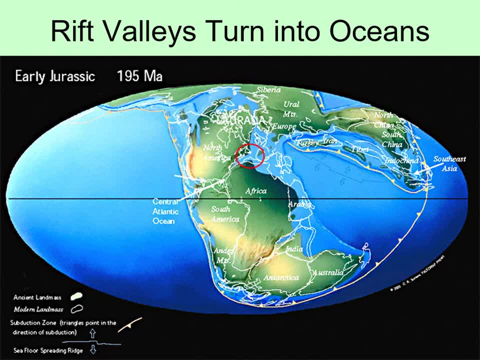 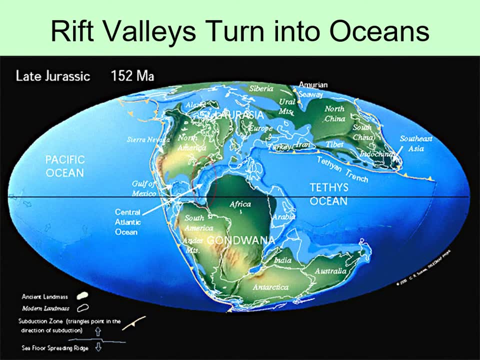 Also, a rift zone is developing on the east side of North America, splitting it off from Africa By 150 million years ago. Europe and Africa have split away from North America, though Africa is still solidly linked to South Africa. Another major rift has developed between East Africa and India. 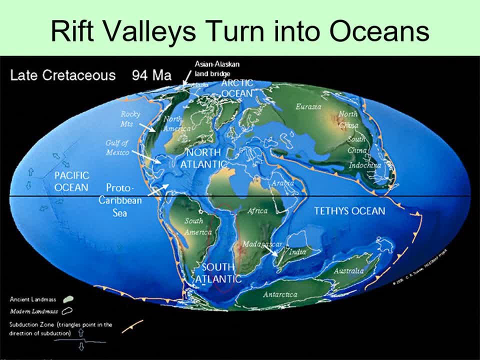 Just over 90 million years ago. a rift between Africa and South America has widened enough to justify the name South Atlantic Ocean. India, Antarctica and Australia have also split off from Africa, and a new shallow sea has developed just east of the Rocky Mountains. 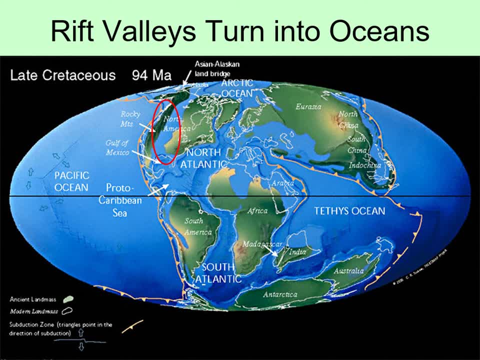 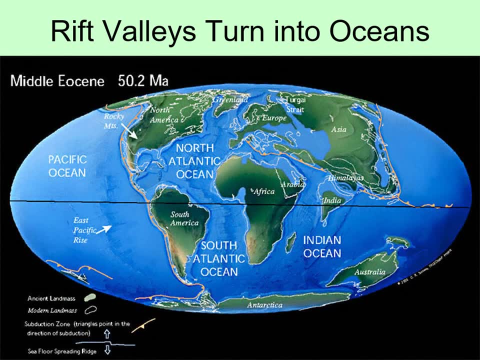 The great dinosaur fossil beds in places like Montana and Wyoming are developing along the edges of this sea By 50 million years ago, after the dinosaurs had died out, the shapes of continents are getting mostly recognizable. The Atlantic is getting wider, though still not as wide as we see today.